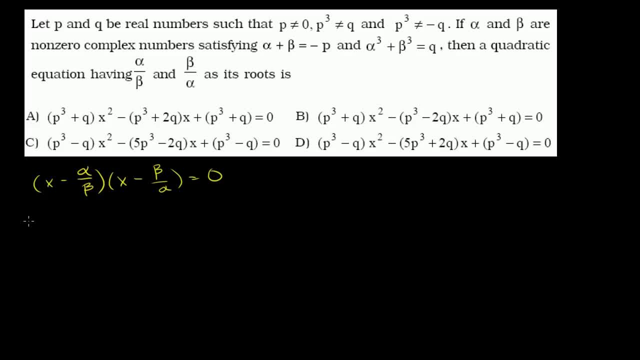 Now let's multiply. Let's multiply this out: x times x is x squared x times negative beta alpha. Beta over alpha is negative beta over alpha x, Then you have negative alpha over beta x, So negative alpha over beta x. And then you have negative alpha over beta times negative beta over alpha. 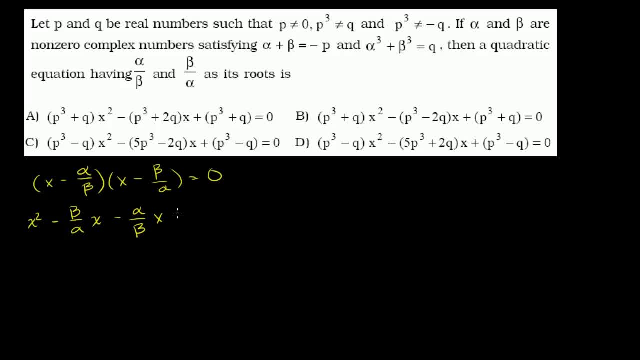 The alphas, cancel out the betas, cancel out the negatives, cancel out And you get plus one. Plus one is equal, is equal to zero. And then let's see- we might be able to simplify this a little bit. If we multiplied, if we multiplied everything times alpha, beta, what will happen? 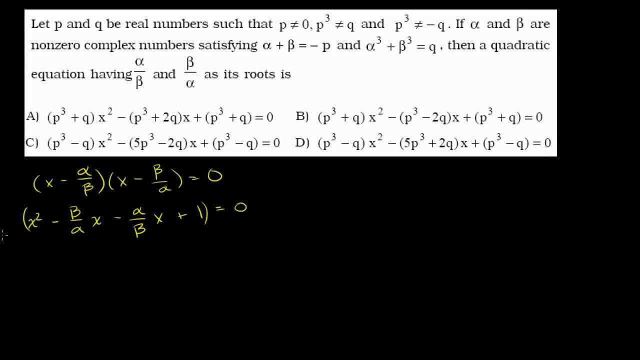 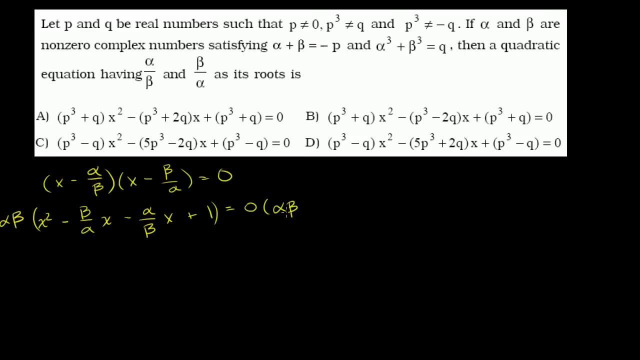 So I'm just going to multiply both sides of. so I'm going to multiply both sides of this equation times: alpha, beta, Alpha beta. I don't like having things in denominators. Clearly, the right hand side is still going to be zero. 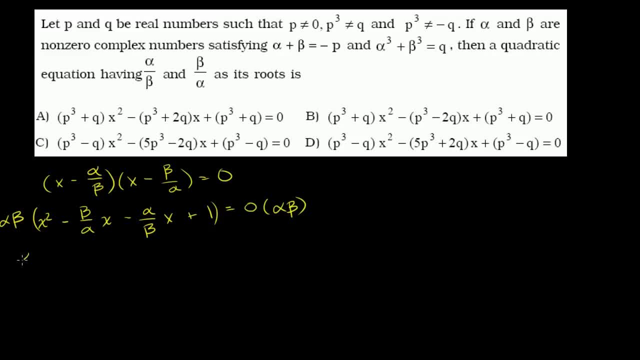 The left hand side now becomes alpha beta x squared. Alpha beta times beta. over alpha: The alphas- cancel out. You have a beta times a beta. So it's negative beta squared. Negative beta squared x Minus the betas- cancel out. 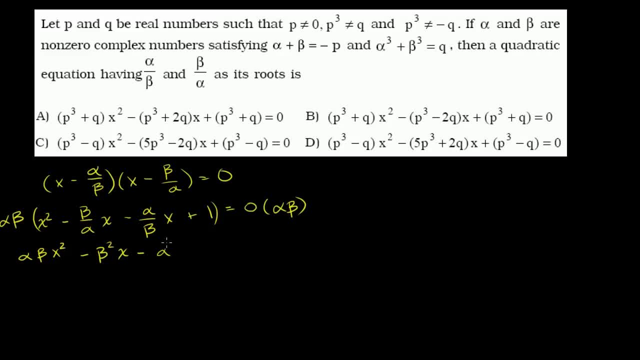 And now you have an alpha times, an alpha Minus, alpha squared x. And now you have plus: alpha beta Is equal to zero, And then we can combine these terms over here. So we have alpha beta x squared Minus, you have a alpha squared plus, a beta squared. 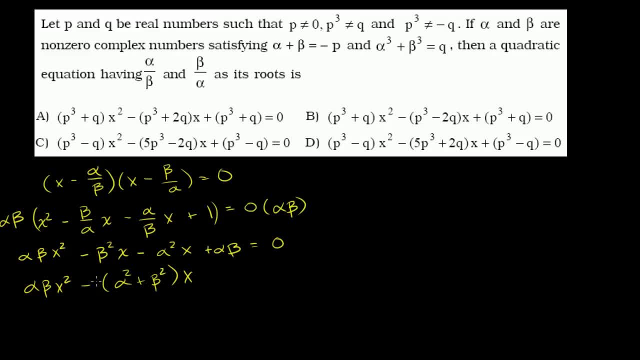 Alpha squared plus a beta squared x. Right, I just took the negatives out of it. Plus alpha, beta is equal to zero. Alright, so everything I did is just kind of you know. I just said, okay, these are the roots. 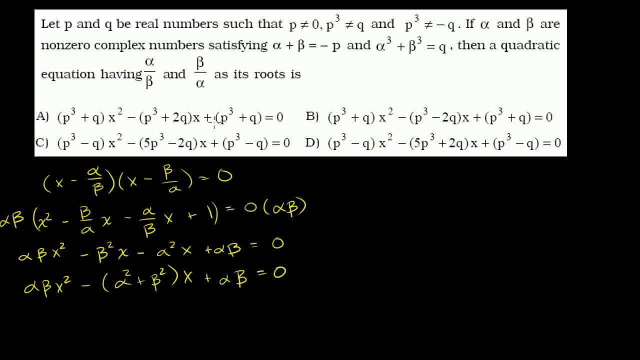 Let me just multiply it out And I got something in terms of alpha and beta. Now, when you look at their choices, clearly they want answers in terms of p's and q's. So let's see if we can convert this into p's and q's. 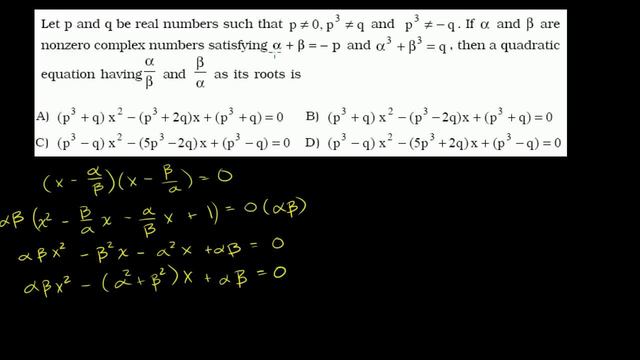 So a good place to start. They tell us that alpha plus beta is equal to negative p, Or negative p is equal to alpha plus beta, And so if we squared that, what I want to do is somehow relate it to q as well. 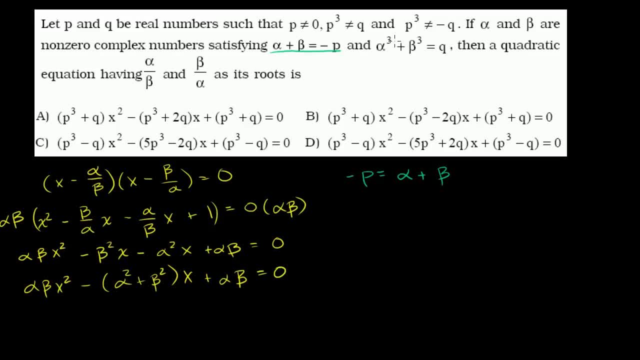 And so maybe if we eventually take it to the third power, we can get some of these terms over here And relate it to q And also, when we square it, I think we'll be able to relate some of these things to it as well. 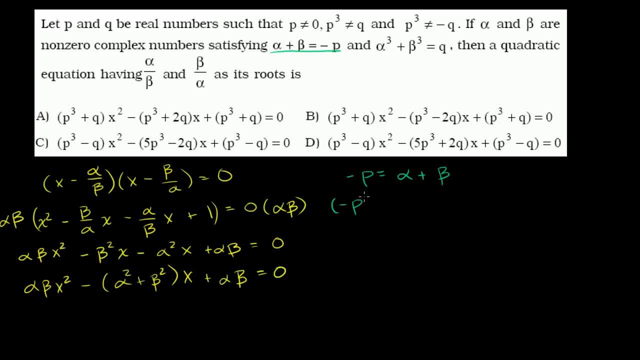 So let's square both sides of this equation So you have negative p squared, which is the same thing. because the negative, let's cancel out. this is the same thing as negative one times p squared, which is negative one squared times p squared. 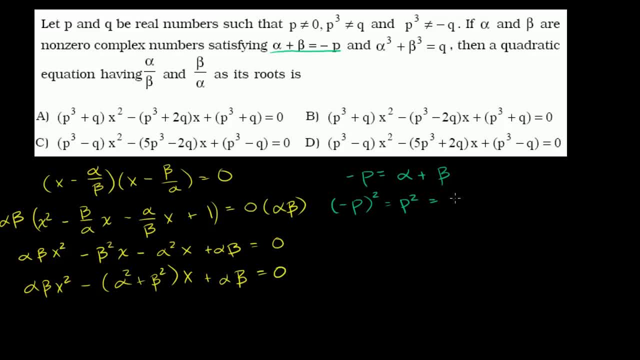 which is just p squared, is equal to this expression over here, squared, which is just alpha squared plus two, alpha beta plus plus beta squared. Fair enough, And already we have something interesting showing up over here. We can express alpha squared plus beta squared. 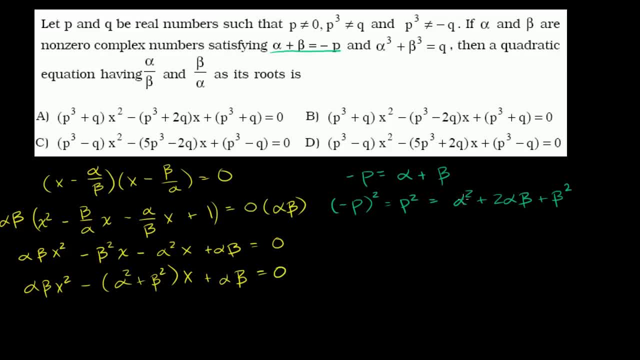 in terms of p squared and alpha, beta. And then we simplify things a little bit. Well, let's just keep going. Let's just take this to the third power. So if we have negative p to the third power, which is the same thing as the negative of p to the third, 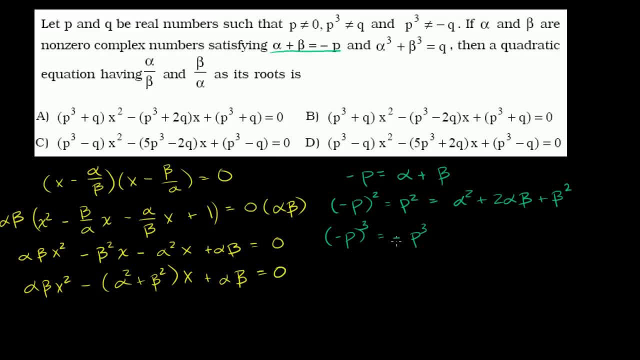 if you multiply this thing times negative p, you're going to get the negative sign p to the third And this is equal to. we could just multiply again. do the distributive property. or, if you kind of remember, Pascal's triangles: 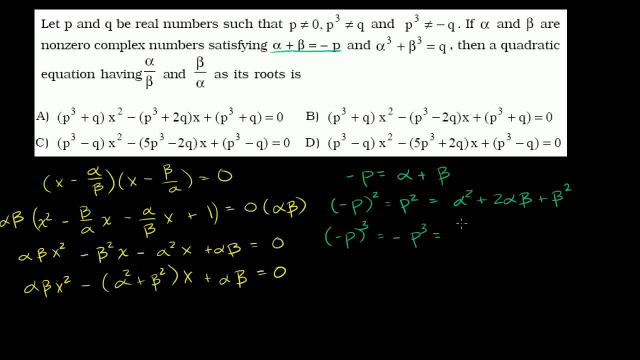 you remember the coefficients on it or the binomial theorem. this would be a faster way to do it. You start with. you know I'll do Pascal's triangle really quick here if you don't want. So you have one, one, one for a binomial. 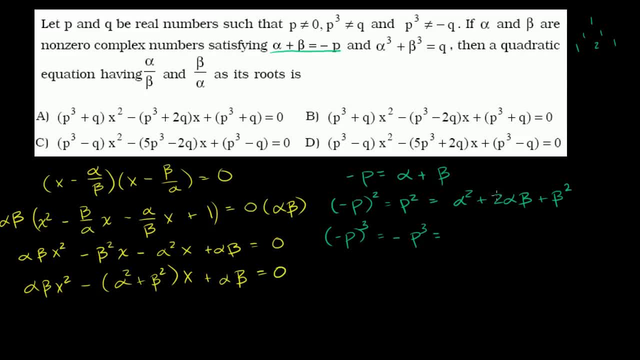 one, two, one. When you take the square of a binomial, one, two, one, And then when you take that to the third, when you go to the third power, it's one, three, three, one. A bunch of videos on this. 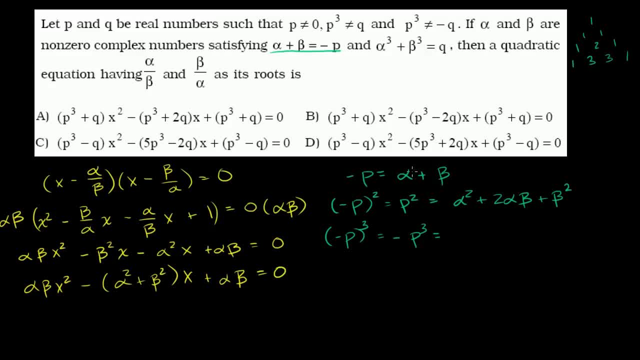 especially in the videos on the binomial theorem. So this to the third power. this thing right here to the third power is going to be alpha to the third plus three alpha squared beta plus three alpha beta squared plus beta to the third. I just decreased the exponent on the alpha each time. 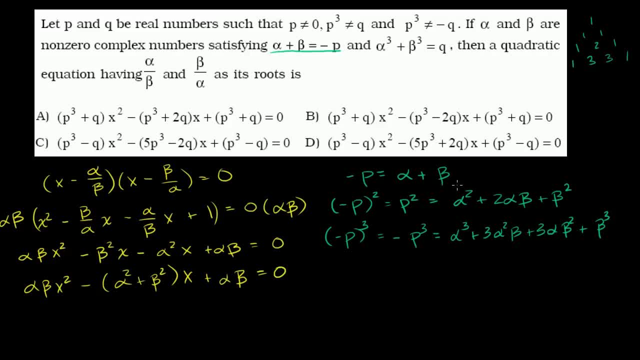 and started increasing the exponent on the beta each time. Or you could just multiply this and you should also get this. And now this is interesting because this is expressing everything in terms of- let's see if we can simplify this a little bit. This is equal to: 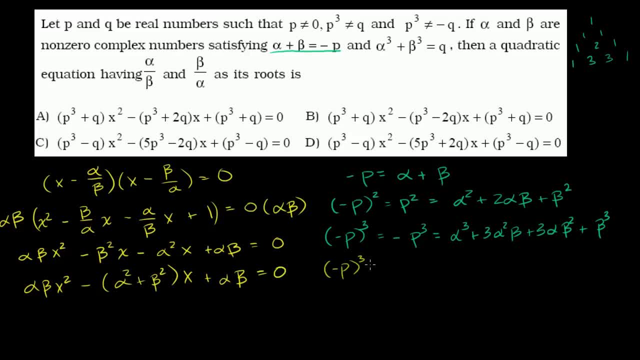 so let me write this: We have negative p to the third, which is equal to negative p to the third, just the difference of the parentheses is equal to. we have this alpha cubed plus the beta cubed, That's those two terms right over there. 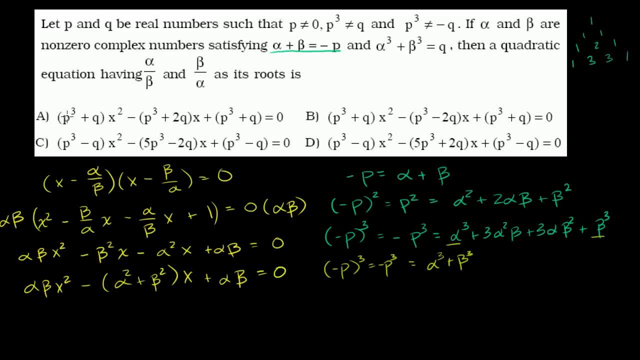 And I separate those out because those are our cubes, Those are our Q. And then I have: let's see over here I can factor out a three alpha beta, So plus three alpha beta. And what do I get If I factor out a three alpha beta here? 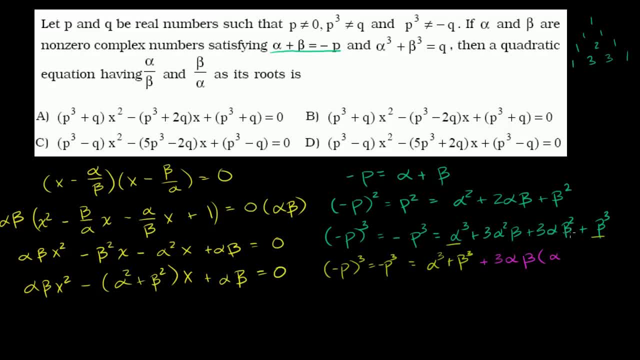 I'm just left with an alpha on this term, And if I factor out a three alpha beta here, I'm just left with a beta. I am just left with a beta. So what does this simplify to? So this is going to simplify to. 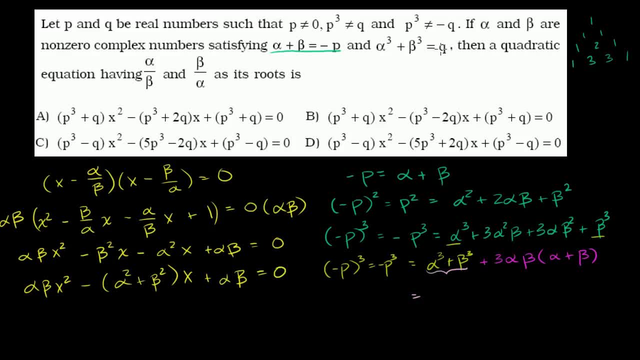 this is going to be equal to this right here is equal to our Q. So this is equal to Q plus three alpha beta. And what's alpha plus beta? Well, they already told us what alpha plus beta is: Alpha plus beta. alpha plus beta is negative p. 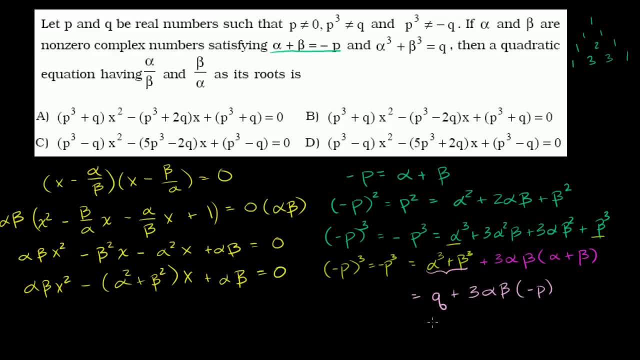 It is negative, it is negative p. So let's see what we can do over here. We have, we can. this right here is the same thing as negative p to the third. So here we can solve for alpha beta, And so we'll have alpha beta in terms of p's and q's. 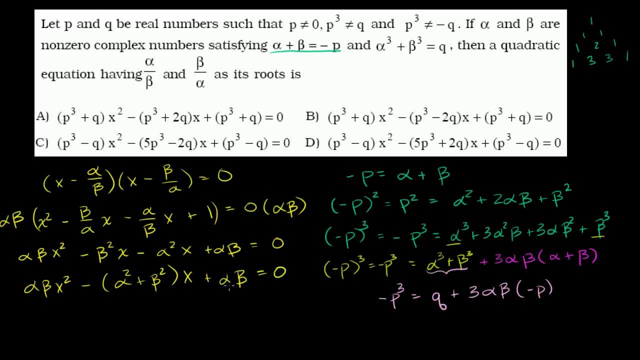 So that'll be good. So we can substitute the alpha betas with whatever we get in terms of p's and q's, And then this thing we can express in terms of a p in an alpha beta, which means we can express in terms of p's and q's. 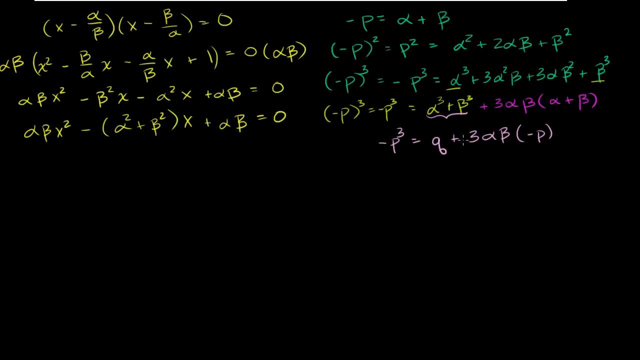 So let me do what I'm talking about. Let me do what I'm talking about. So let's just solve first of all for alpha beta. So if we solve for alpha beta first, we want to subtract q from both sides of this equation. 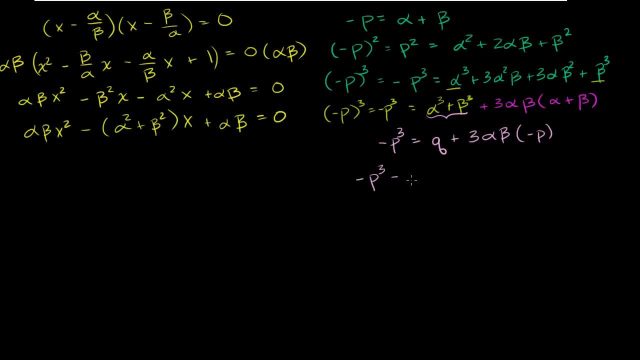 So you have negative p to the third minus q. minus q is equal to- we have this negative sign over here- So it's equal to negative three, alpha beta p, And I want to solve for alpha beta. So let me divide both sides by negative three. 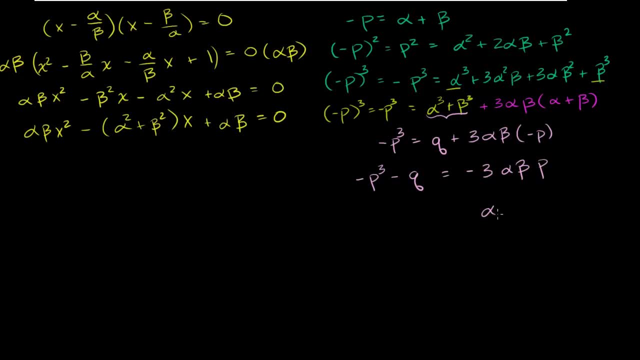 And so we get on the right hand side, we get alpha beta. alpha beta is equal to: if you divide- let me just write it out because I don't want to make a careless mistake- So you have negative p to the third minus q. 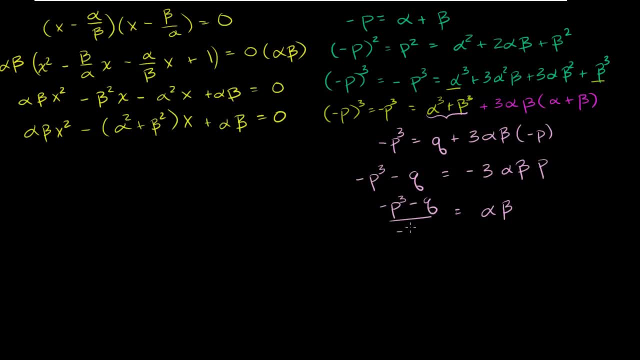 over negative three p Over negative three p. Now, if we multiply the numerator and denominator by a negative sign, we get p to the third plus q over three. p is equal to, is equal to alpha beta. So we can now express this and this term in terms of p's and q's. 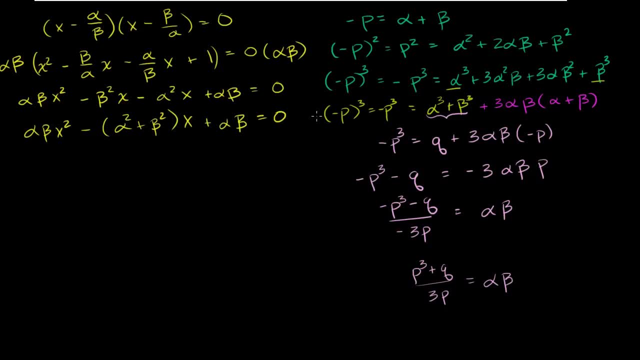 Now what about this one right here? So what is alpha squared plus beta squared? And we see right up here alpha squared. that's alpha squared plus beta squared. So if we subtract two alpha beta from both sides of this equation, we get alpha squared. 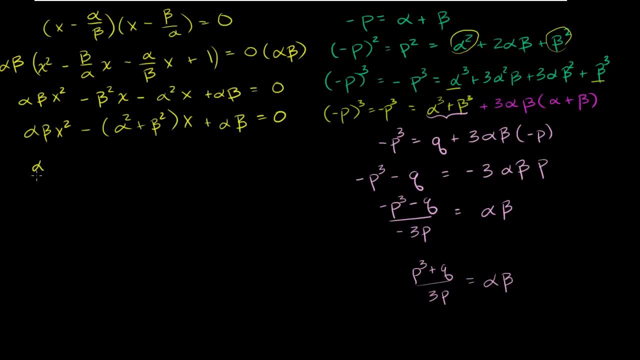 alpha squared plus beta. let me do this in a different color We get. we get alpha squared plus beta. squared is going to be equal to p. squared is equal to p. squared minus is minus two alpha beta Minus two alpha. 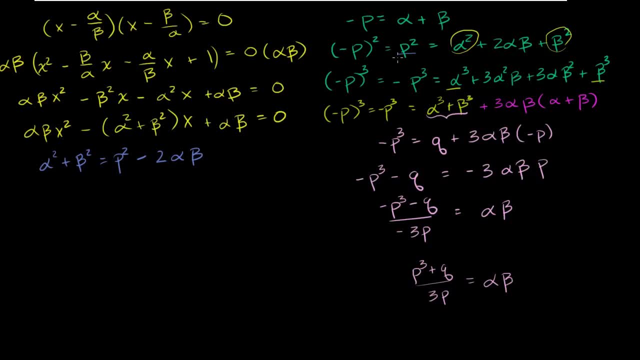 minus two alpha beta. Right, I just subtracted two alpha beta from both sides, And so this is going to be equal to p squared minus two times this thing, Minus two times p to the third, plus q over over three p. 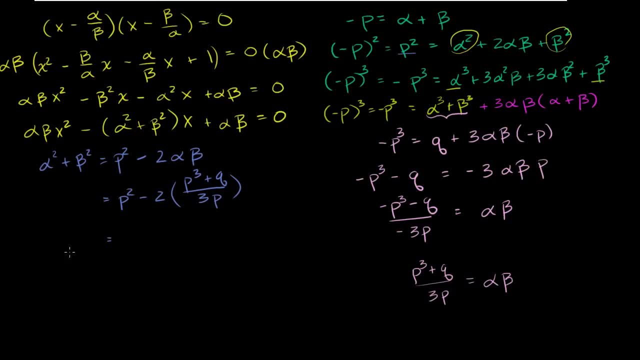 Over three p. And what is this equal to? This is equal to: let's put on a common denominator: p squared over, this is the same thing as three. my cell phone rang. I had to pause it, sorry. So this is equal to three. 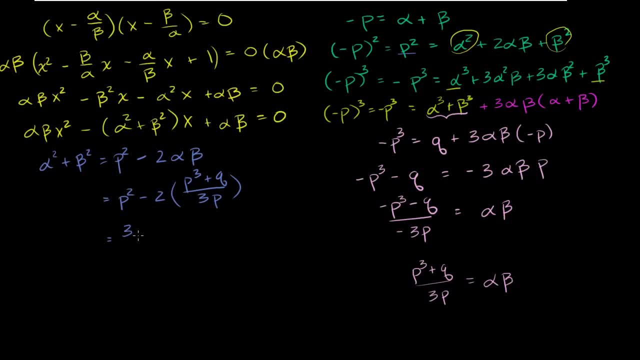 three p to the squared. if I want to put it over, three p is equal to three p. three p to the third, over three p. Let me make it clear: This term right here is this term over here, If you were to simplify it. 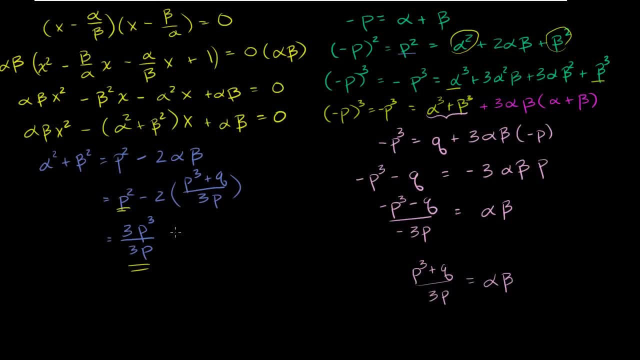 threes cancel out. you'd just have p squared And then you have minus. I'm just going to distribute the negative two minus two p to the third minus two q, all of that over three p. So it is equal to three p cubed minus two p cubed. 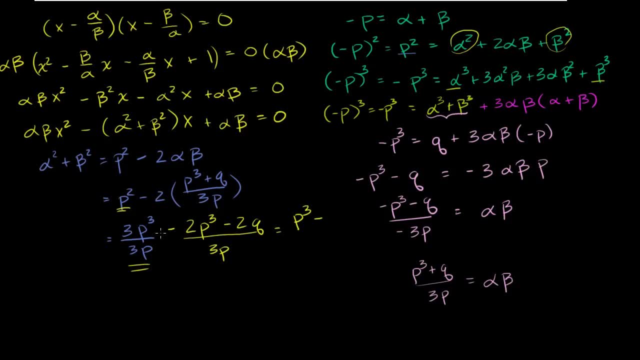 is equal to p cubed minus p cubed minus two q minus two q, all of that over three p. So now we have- we can write this entire expression in terms of p's and q's, This first term over here. 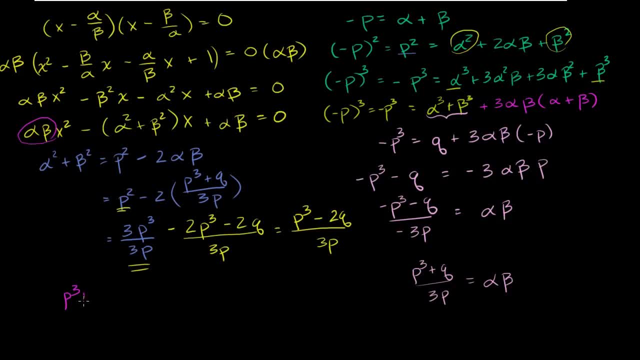 alpha beta. this is p cubed plus q over over three p, And we want to multiply that times x squared, x squared, And then you have minus, minus, alpha squared plus beta squared. We just figured out that alpha squared plus beta squared 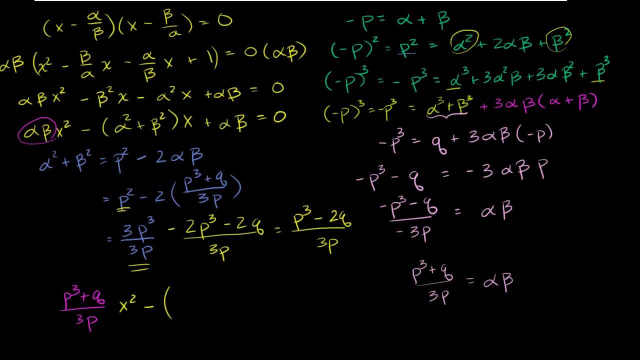 is this thing over here. So minus, I'll do it in a different color, I'll do it in green. Minus this thing. p to the third, minus two q over three p over three p, And that's going to be multiplied by an x. 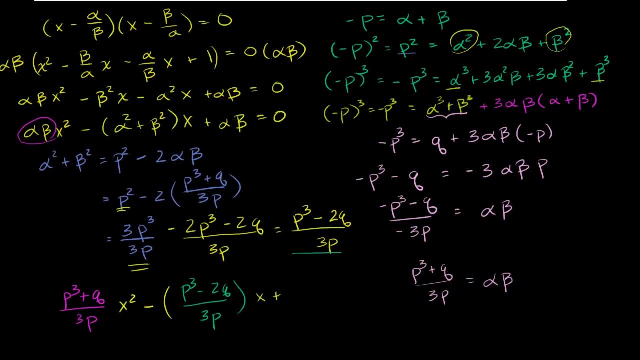 By an x And then plus alpha beta again. So alpha beta is p to the third plus q over three p. Now when we look at any of the choices up here, it looks simplified. We don't see any three p's in the denominator. 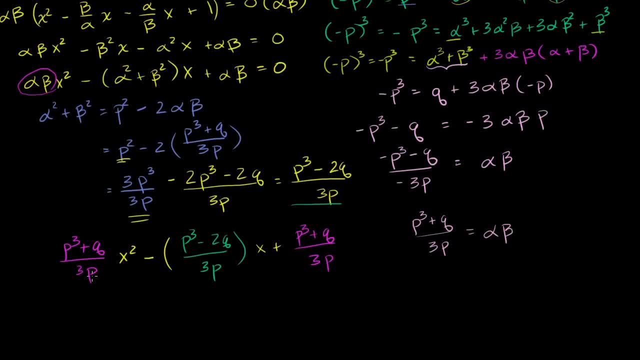 So let's see if we can simplify that. If we can simplify that, If we multiply this: oh, and we won't want to lose, We had an equal zero here the whole time, So this is equals zero. So you multiply both sides of this equation by three p. 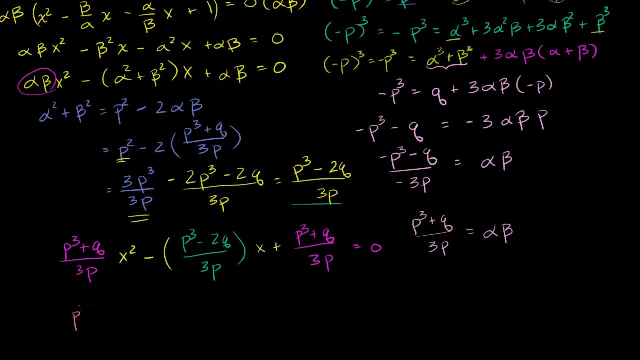 What do you get? This first term becomes p to the third plus q times x squared. The second term becomes minus p to the third, minus two q x. And then this last term becomes plus p to the third, plus p to the third, plus q. 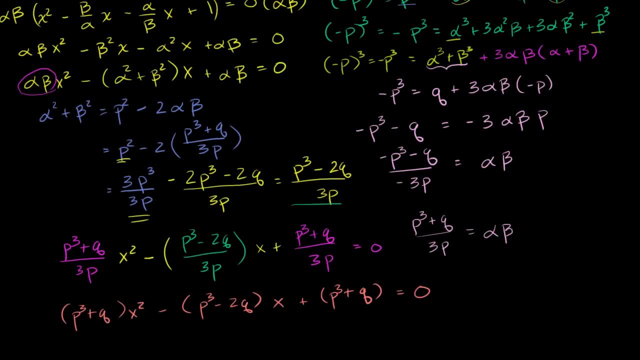 And this is going to be equal to zero. So let's see how this compares to the choices, And I think I actually did not make my careless mistake in this video. I actually got the right answer. Let me see. It shows you when you do it carefully.